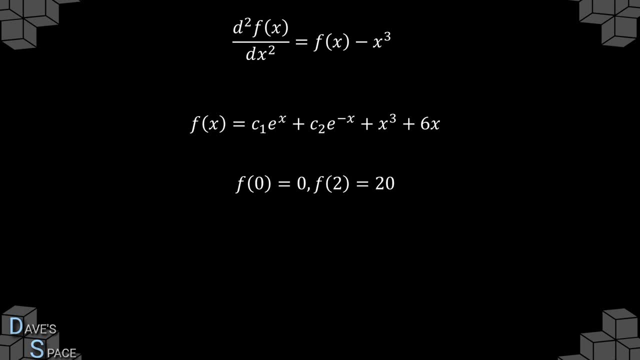 condition which gives more information about the equation, The boundary conditions here, which is the solution to the equation at two points, provides enough information to remove the constants of integration. Here we are given: the function evaluated x equals zero is equals zero. The function evaluated x equals two is equals 20.. After some math it is found the solution. 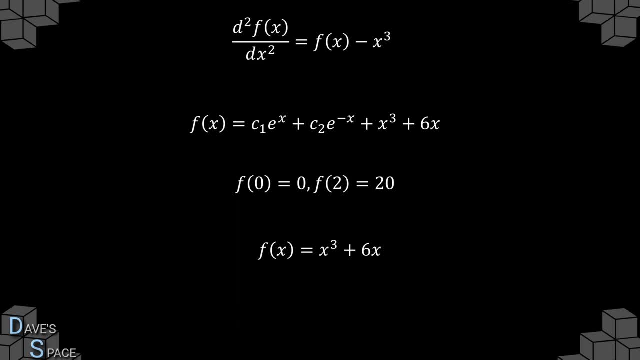 to the equation is x cubed plus six x, which is unique. There are no unknown constants in this equation. This is known as the analytical solution. It means that the function of f can be evaluated at any point in space x. But what happens if we are not skilled enough? 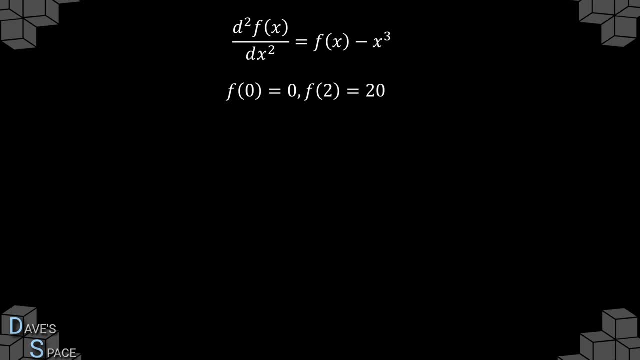 to solve the equation Or, even worse, an analytical solution does not exist. This is where we can use the finite difference method. Here we define a domain in which we evaluate our solution. Here we choose zero to two, since the conditions given were between zero and two, Or, more specifically, the extra information. 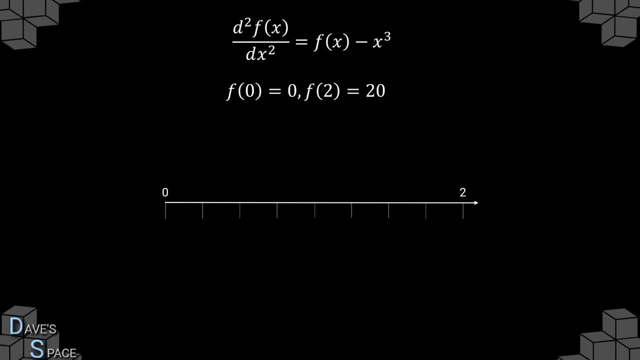 we were given is that the function at zero is equal to zero and the function at two equals 20.. We then divide up this domain into small chunks. Here we have uniform chunks of length h. These are chunks of finite difference. We will then evaluate the function at discrete points. 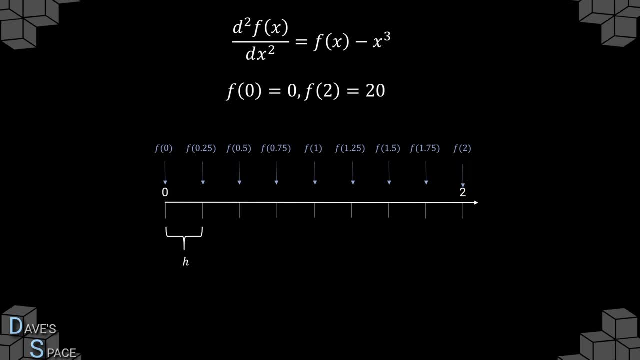 or nodes. So how do we go ahead and solve this equation? Well, let's take a step back and look at how we can define a function. The Taylor series allows us to estimate the value of a function at a point x plus h. We use evaluations of the function f of x and its derivatives to 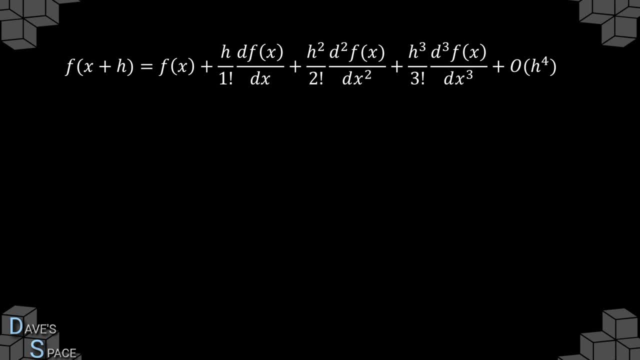 evaluate the function of f of x plus h. The big O notation here It's used to say that any terms not written out at the fourth power of h or higher. Now what happens if we evaluate this function at x minus h, x and x plus h and multiply? 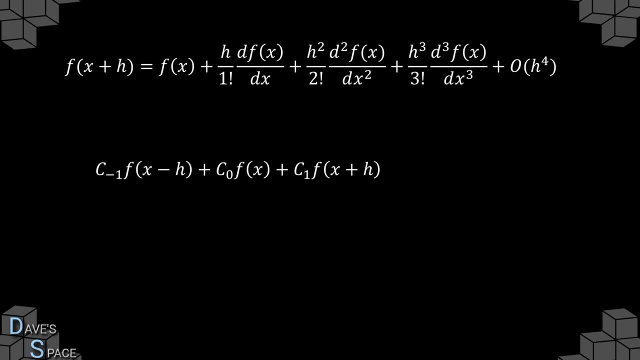 them by some constants: c minus one, c and c plus one. It turns out that it is possible to find coefficients such that the sum on the left is equal to the second derivative of the function f of x. Plus are terms proportional to h squared, and the constants that satisfy this condition are given. 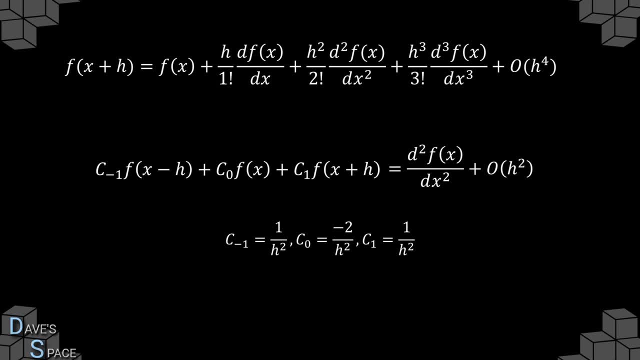 here, with c minus 1, c 1 being 1 over h squared and c 0 being minus 2 over h squared. this gives us a following equation: notice here how we are left with terms that are proportional to h squared and higher. but what you notice here is that we now have a way of evaluating the second differential. 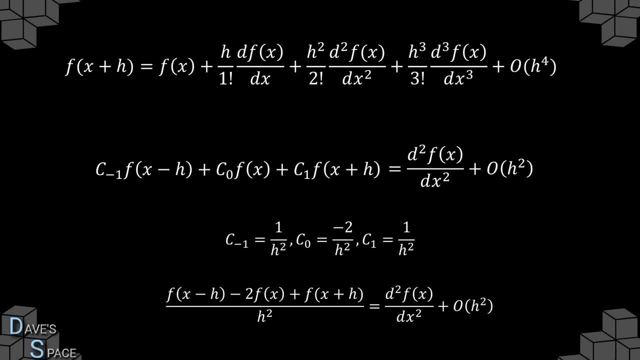 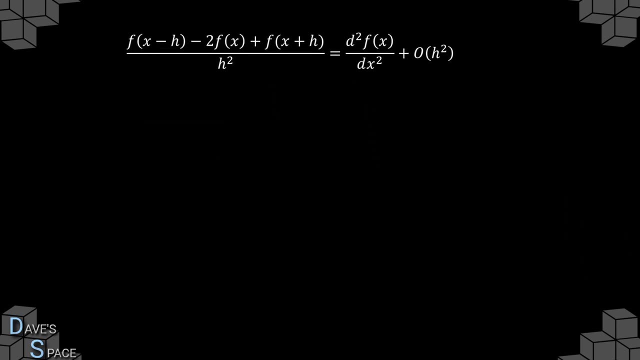 of a function d squared, f of x over dx squared, as an evaluation of f of x at three points: one at f of x, one at f of x minus h and one of f of x plus h. if we then drop the higher order terms, it's part. 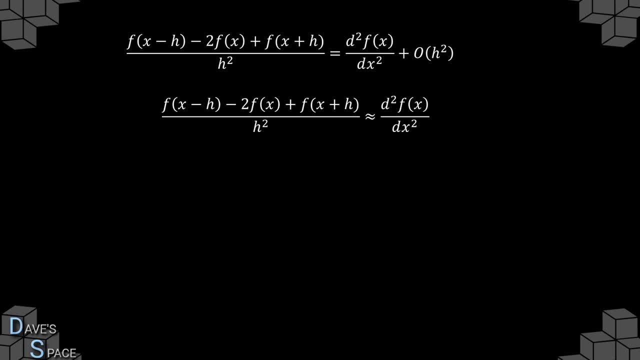 of the big own notation, we can use it as an approximation to the second differential. we now have an equation that relates the second differential, point x, to the function evaluated at neighbouring points x plus h and x minus h, which, as noted earlier, are a finite distance away, and so we have completely removed the differential term. 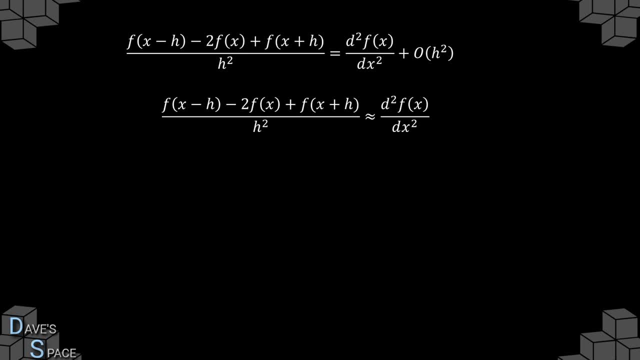 This is the key point of the finite difference method. We transform differential terms into equations that only use the function evaluated at different points. Some of the astute viewers may recognise this equation as if this equation is taken to the limit where h equals zero. 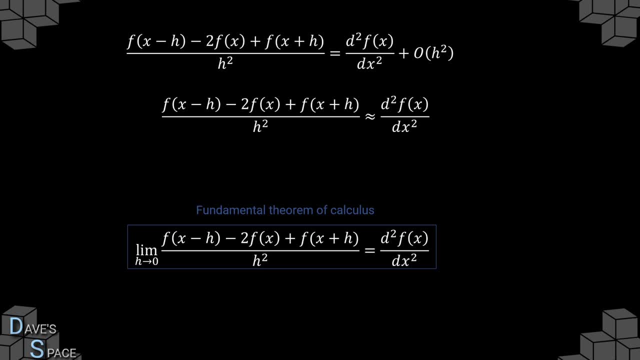 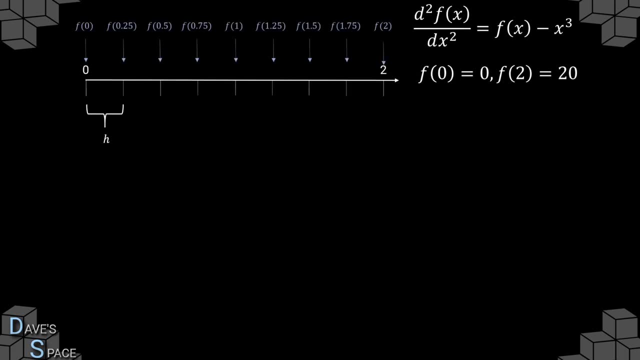 and you get the fundamental theorem of calculus with the second differential. So, going back to our original example, if we split the domain of zero to two into eight chunks or nine points, this will give us a spacing of h equals 0.25.. We can evaluate the function. 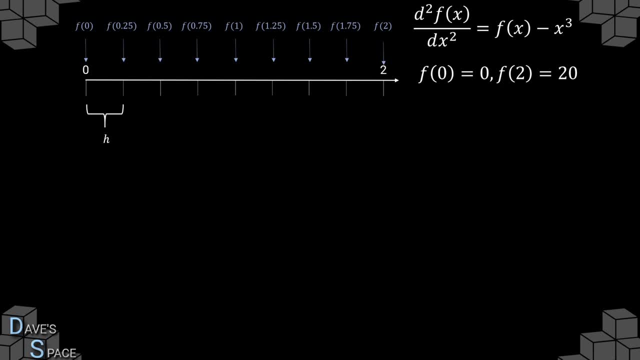 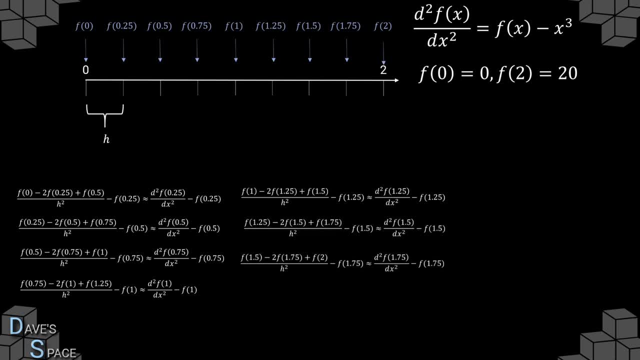 points of our system. We haven't evaluated the function at zero or two, because we already have this information in the form of boundary conditions. So how do we actually solve this? Well, you may notice that we now have nine equations and nine variables we need to solve for. 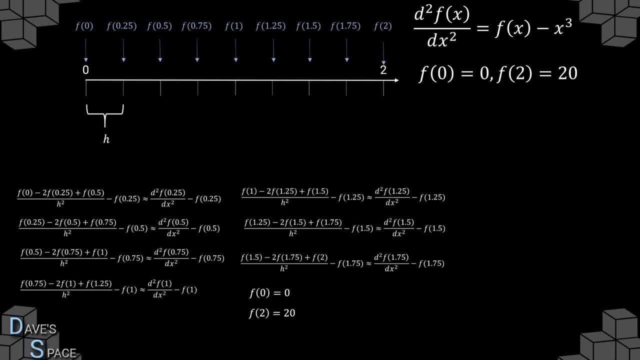 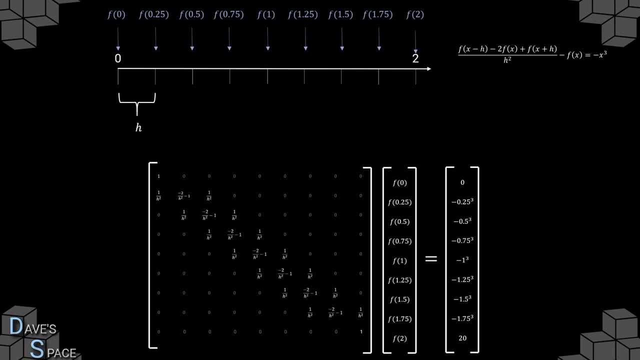 The nine variables are the function evaluations at each of the grid points, and so we can express these equations as a vector of f values. We can then arrange the equations to show, and this matrix on the left contains all the simultaneous equations and the vector on the. 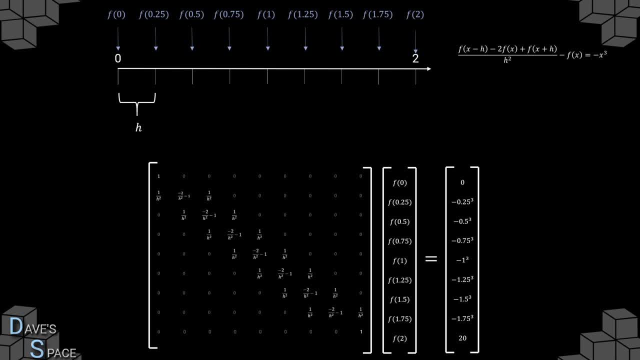 right contains all the solutions to each row of equations. We can see the boundary conditions are in the equation matrix and the vector on the right. So the top left of the matrix has a 1 in the first column, corresponding to the boundary conditions, and the vector on the right contains all the. 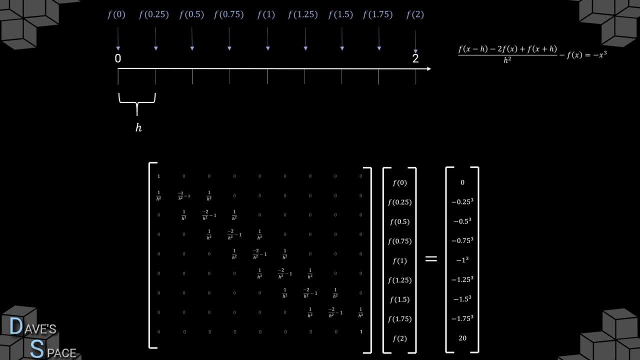 boundary 0, the one in the bottom row, in the column to the farthest right, which represents our boundary of 20.. So this matrix system completely describes all the equations we derived previously, And this matrix is in the form: A times F equals B, with A being the matrix, F being the solution and B being our individual. 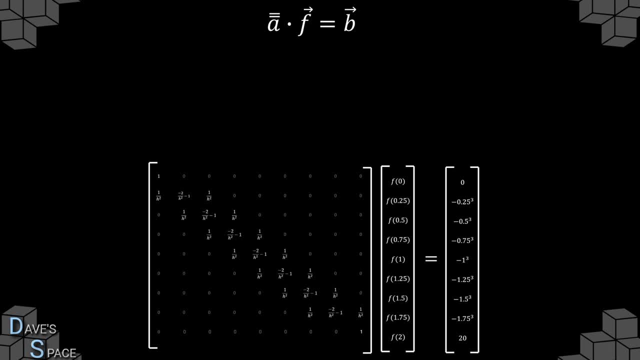 solutions for each of the equations in A. We can solve this by taking the inverse of matrix A and pre-multiplying equation B to give us our final answer. This method is known as a direct method, as a solution F is found by solving the. 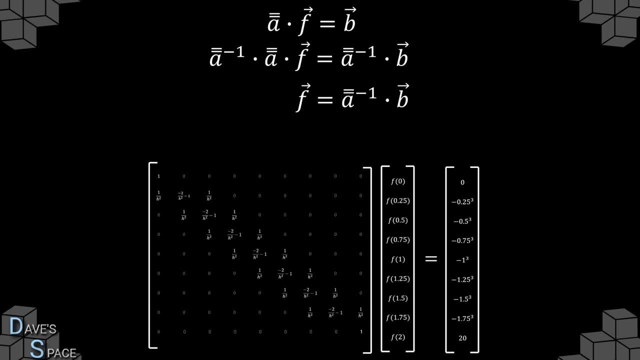 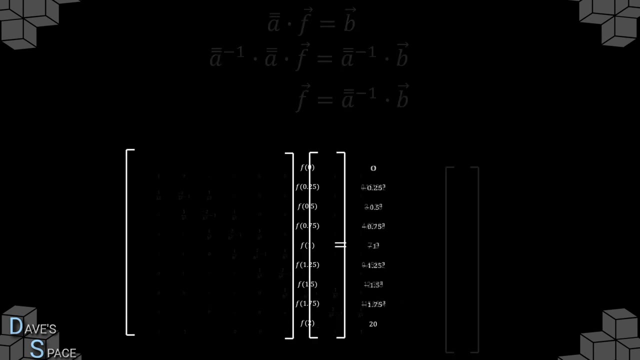 equation directly. It should be noted that as the number of grid points become larger, the size of the matrix becomes square as large. For large matrices, it is often more practical to use sparse matrices and sparse solvers to limit memory usage, since most of the elements are zero. 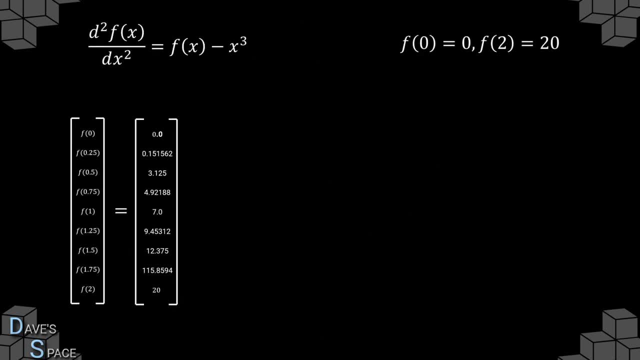 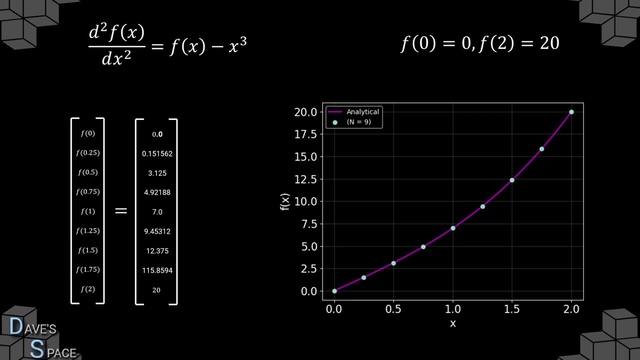 The solution is then the function evaluated at the points with second order accuracy. The solution does not tell us the analytical solution to the original differential equation, but an estimate to the solution evaluated at those specific grid points. This is indicated on the plot on the right, where the points are the values given from the finite difference. 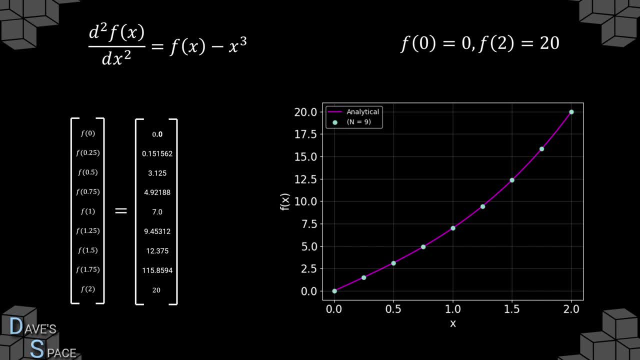 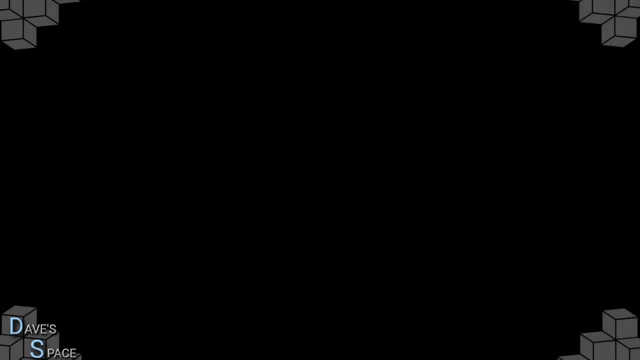 equation and the curve is the analytical solution that we know to this equation. Remarkably, the finite difference approximation for this differential equation returns the exact solution evaluated at the grid points. Why is this? Going back to our original series and using the known analytical solution, we 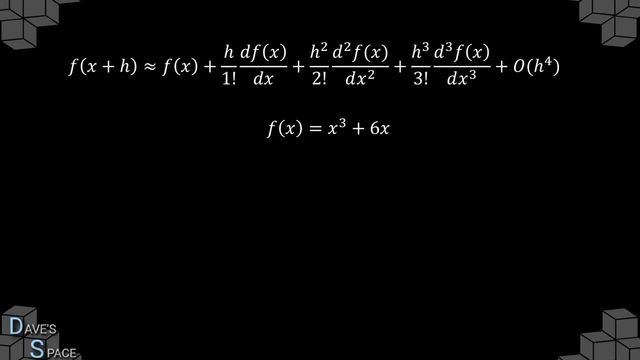 can see that any higher-order terms higher than h power 3 do not remain. Hence our finite difference approximation gives the exact solution. This is not always the case, however, And so, to recap, the finite difference method can be used to solve any ordinary differential. 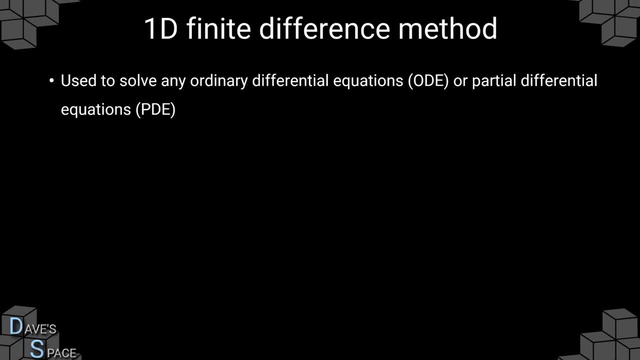 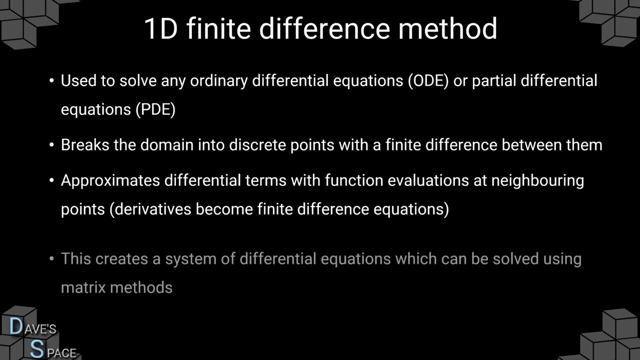 equation or partial differential equation. It breaks down the domain into discrete points with a finite difference between them. It approximates differential terms with function evaluations at neighbouring points, that is to say, derivatives become finite difference equations. This creates a system of differential equations which can be solved. 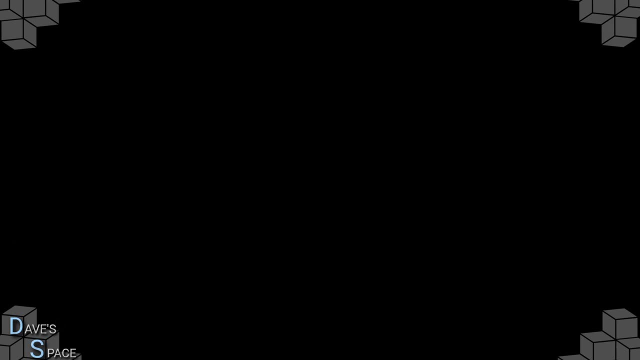 by using matrix methods, And so, moving on, one thing to note is that we use the central difference approximation in converting the second order differential term into a linear combination of function evaluations at neighbouring points. We could instead have chosen to find coefficients that allow for second differentials at a point to be approximated at only point. 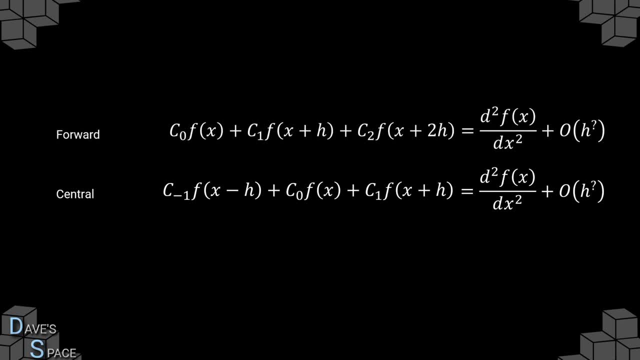 to the right of the current point. This is known as the forward difference. so the evaluation of the second differential of f of x only depends on the value of f of x and points to the right x plus h and x plus 2h. We can also extend this and only look at points on the left, So here: 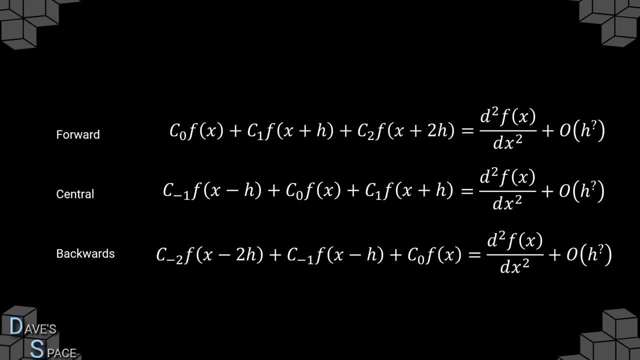 the second differential of f is evaluated using the function at f of x and two points to the left of it: x minus h and x plus 2h. So that's the directly related function. This is divided into minus 2h. all together these are known as the forward, central and backwards finite difference. 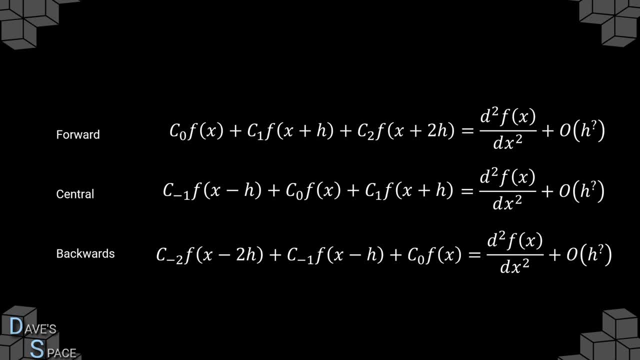 method. it's not always straightforward finding these coefficients for a given accuracy. instead, the coefficients for a given number of terms are calculated and then the accuracy is found from the remaining terms. so in this example, once working through the math, you see that the forward and backwards finite different methods return an accuracy of h to the. 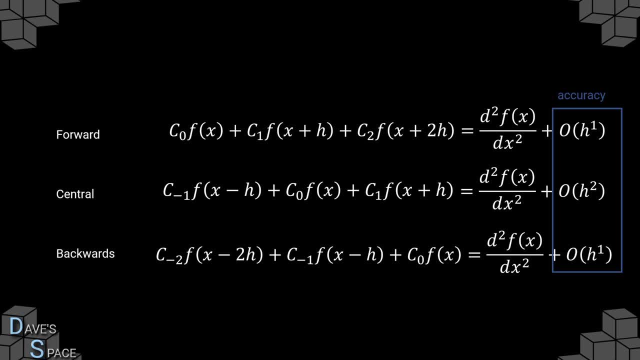 one, whereas the central difference returns an axis of h squared. and you'll notice, we've used the same number of coefficients for the forward, central and backwards, but the central, finite difference- approximation- returns much better accuracy. that is to say, the only terms that remains are proportional to h squared, and there exists tables that can be used to look up the 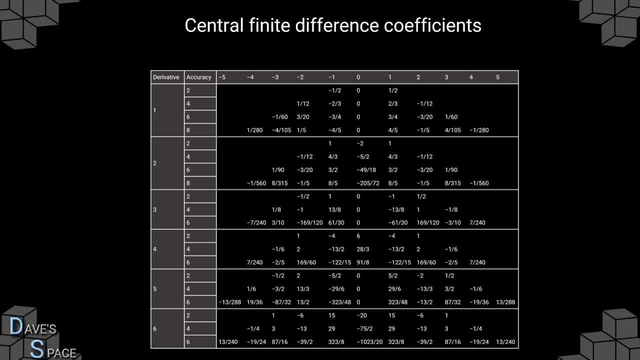 required coefficients for the central, forward and backwards finite difference. approximation and backwards finite different methods for a given derivative. along with the accuracy of the method. here we have the central difference table for a given derivative, which is on the left hand side, and accuracy: the number at the top indicates which terms to evaluate, for example, x, x plus h. 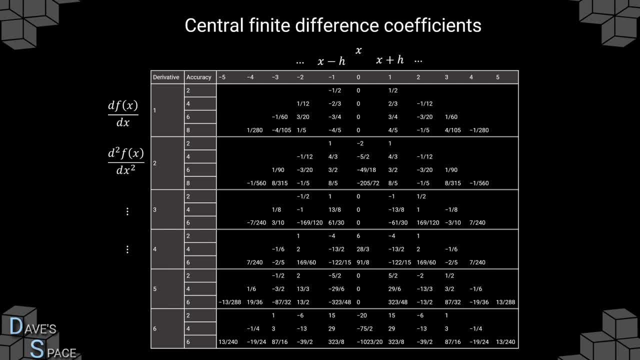 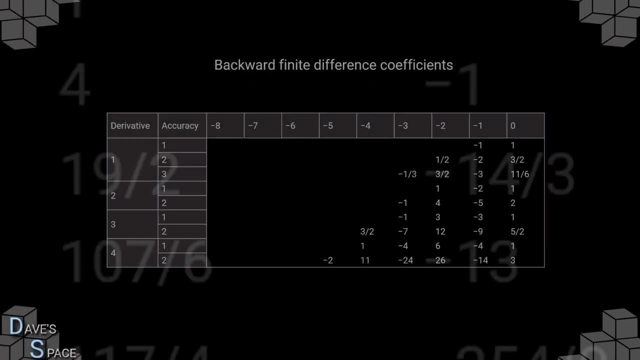 x minus h, etc. the number associated with the derivative indicates the power of h to divide by, and accuracy is the lowest power of h that we ignore when setting up the equations. here are the coefficients for the forward finite difference method. here are the coefficients for the backwards finite difference method. 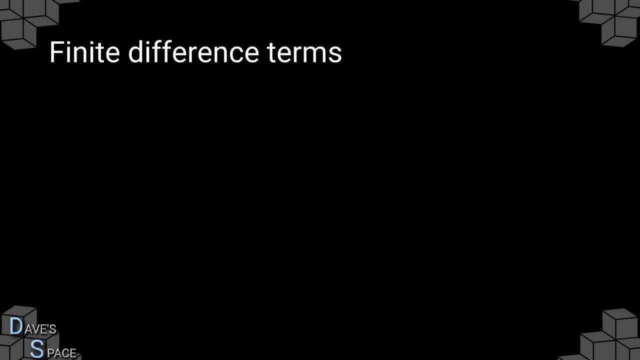 and you don't necessarily have to stick to the tables either. in general, more coefficients equals better accuracy, as more information about more points is used to calculate the derivative. but just remember: the approximation is only as accurate as the lowest order. so let's consider the following problem. solve this equation in the domain of x equals 0 to 3.. 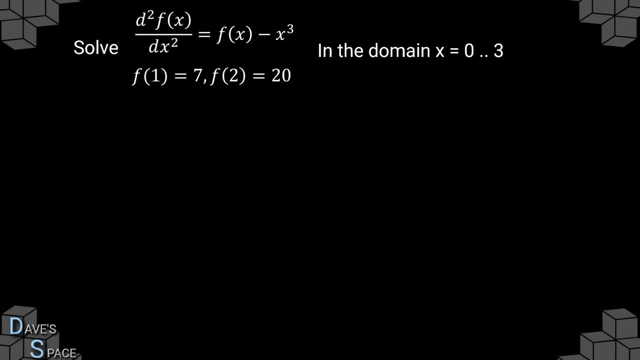 so you see, now we've been asked to solve the equation between x equals 0 and x equals 3, and we're giving two internal points. so these are no longer boundary conditions, these are points in the middle of the equation or, more specifically, in the middle of the domain to which we've been. 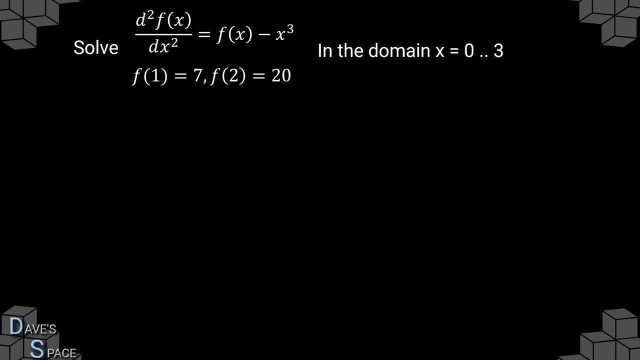 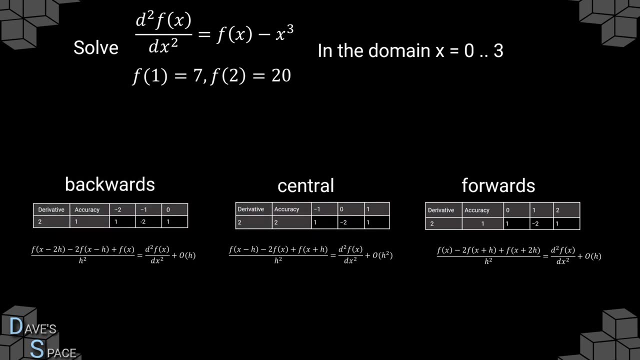 asked to evaluate it and let's see how we can use both the forward, backwards and central finite difference methods to actually solve this equation. we will choose three coefficients for each method, which gives a first order accuracy for the forward and backwards method, and the second odd accuracy- the central difference method. 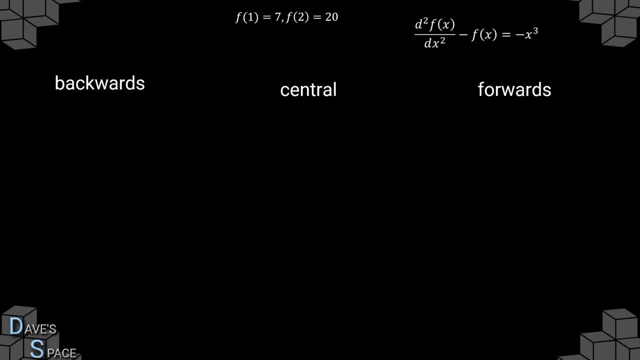 so we will set h equals 0.5 for now, which gives us seven points. so we will set h equals 0.5 for now, which gives us seven points. This will then give us the following matrices for each method. It also gives us the following points for our internal boundaries: 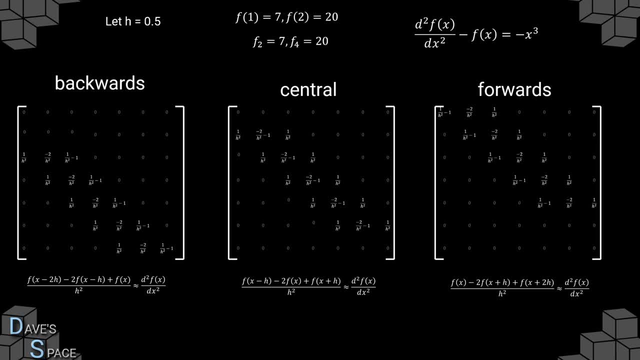 Here we have used index notation to find that the third index corresponds to x equals one, and the fifth index corresponds to x, equals two. remembering that indices start from zero, We can see that the location of the minus one term that comes from the equation and the row in which the equation sits is the only difference between the matrices. 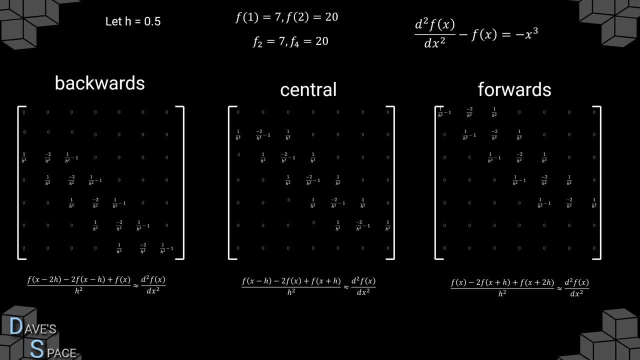 We can see that we can comfortably fill the matrix for all but two of the rows. All that's left to do is input the boundary conditions. When we insert the boundary conditions into these matrices, we get square matrices which can be solved via decomposition. All we need to do now is find the expression for the b vector. 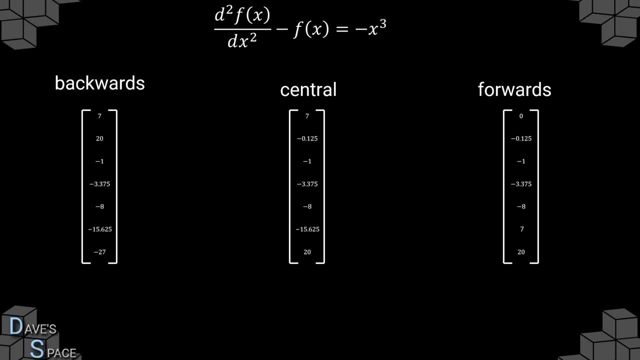 Ok, We can see here that the b vector represents the right hand side of the differential equations, or the equations to which we use the finite difference approximation to turn the differential into a linear sum of adjacent points. We can see that the b vector represents the right hand side of the differential equation. 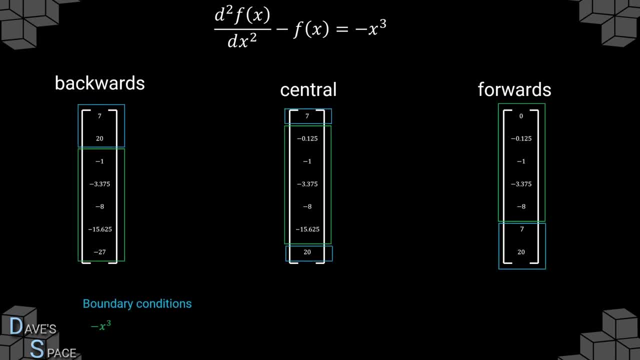 but the boundary conditions inserted in the rows in which the finite difference approximation would not fit. It doesn't matter that the boundaries are not in order. A key point with matrix decomposition is that the rows can be swapped freely from the a matrix as long as the corresponding rows in the b matrix are swapped. 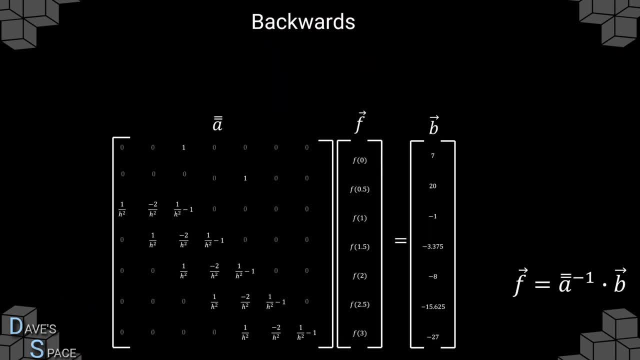 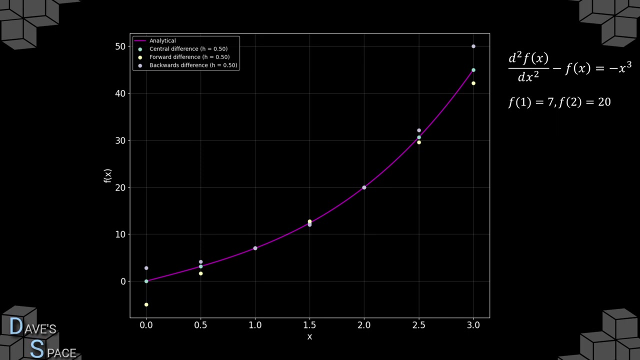 The solution will always be the same, And so the expression for the backward system of linear equations looks like this. Likewise for the central- finite difference method looks like this. Likewise for the forward- finite- Ok, finite- difference method looks like this: And here is where the difference between 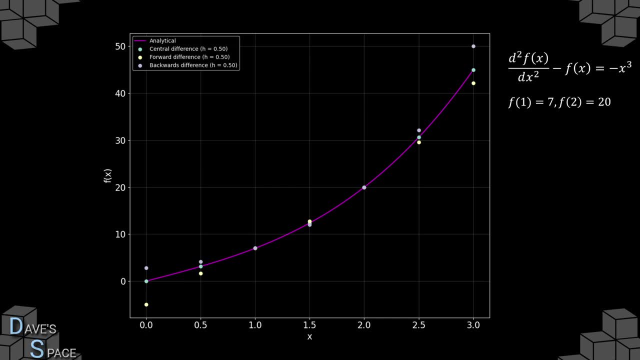 the methods becomes apparent. We have here the solution for the forward, backwards and central differences. The forward difference underestimates the solution outside the given boundaries and overestimates the function inside the given boundaries. The backwards difference overestimates the solution outside the given boundaries and underestimates the function. 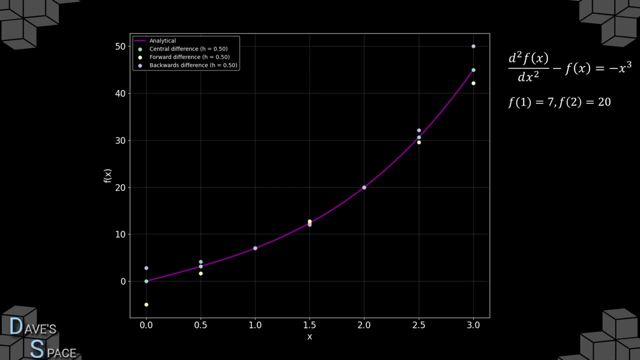 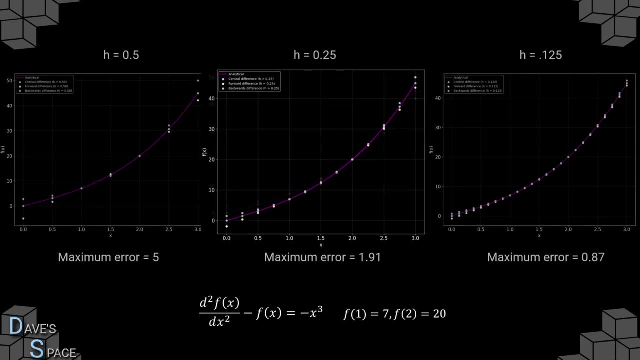 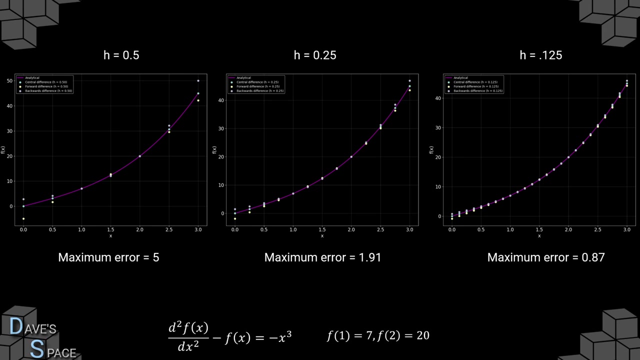 inside the given boundaries. As we saw earlier, this differential equation is solved exactly by the central difference approximation, And if we change the step size h, we can see how the approximation changes. The error from the finite difference approximation is reduced. with reducing step size We can see that the error reduces approximately linearly. 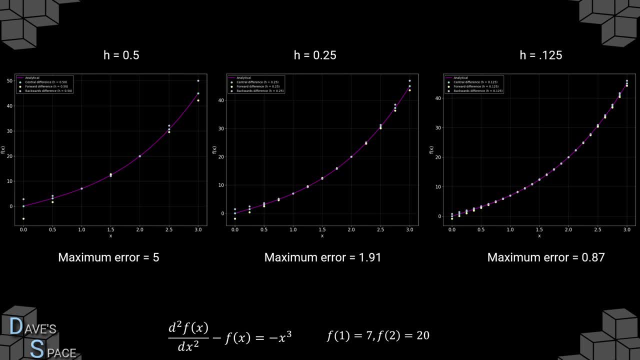 due to the forward and backwards differences being proportional to step size h. These errors are the local error maxima, that is to say, how far is the furthest point from any of the methods, from the analytical solution? is It's clear from this that the 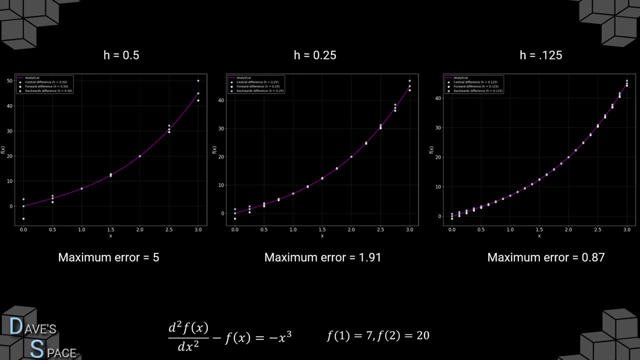 central difference approximation is superior to both the forward and backwards differences. If we use a higher order finite difference method, we can reduce the local error to be proportional to the higher power of the step size. So how do we implement higher order approximations? 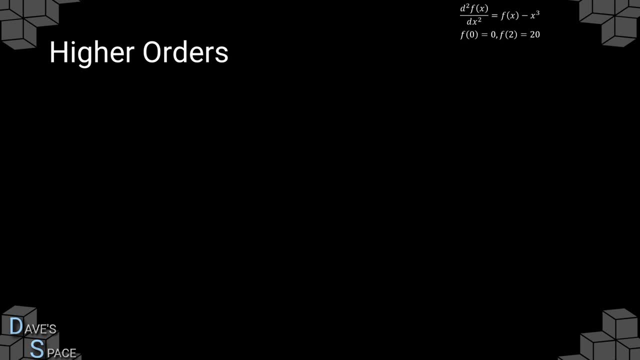 So, if we recall, earlier, we had a boundary value problem in which we were given two boundaries. This is the most common type of problem that you will face, since quite often a solution is known only at the boundaries. Our use of the second order equation allowed us to generate 7 out of the 9 equations required. 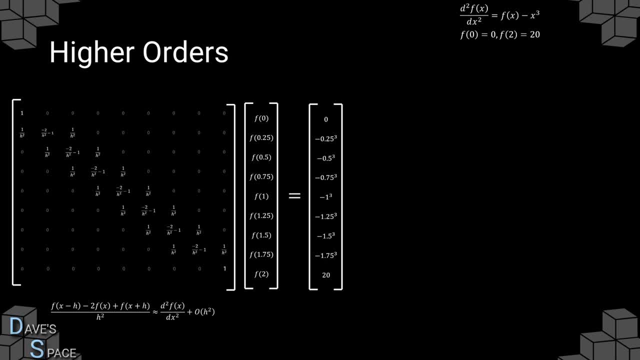 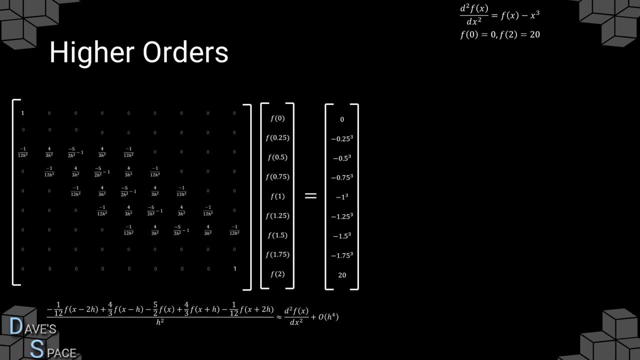 with the last two coming from the boundary conditions. What if, instead, we wanted to use higher order equations, higher-order approximations, say one in which we have an accuracy of 4,? we no longer have enough equations to solve the system. We can see there are two rows. 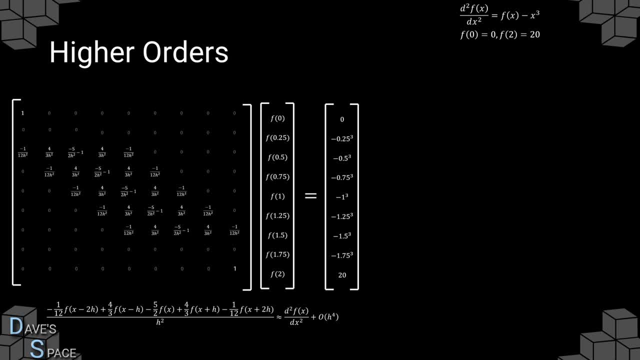 missing from our matrix, as the higher-order approximation doesn't fit within these missing rows. Also, problems like this will rarely offer more points in which to find a solution, since this is a boundary value problem, meaning we only have two points given to us at the boundaries, which, for one dimensions, 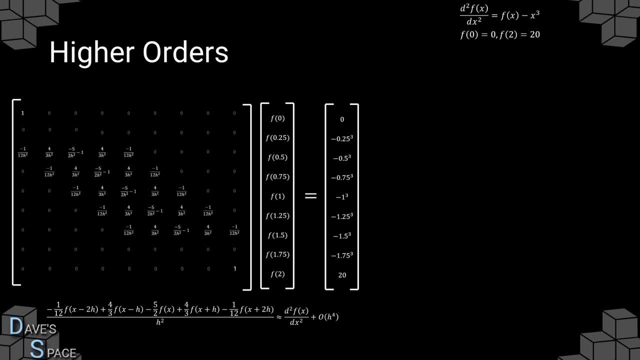 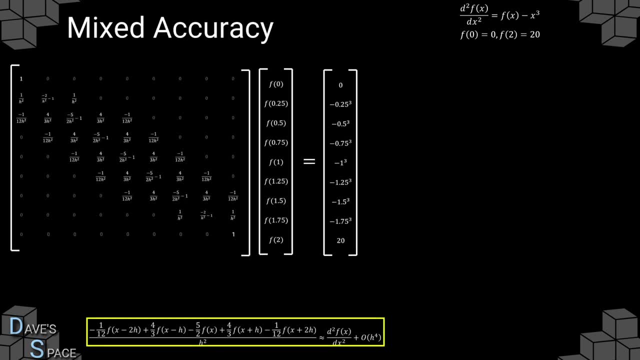 means two points. So to solve this we have two options. The first way is to keep our fourth-order equations and then subsequently use lower accuracy at the edges. So we're fitting in the equations in which we have h to the squared accuracy in the rows in which we have two points. 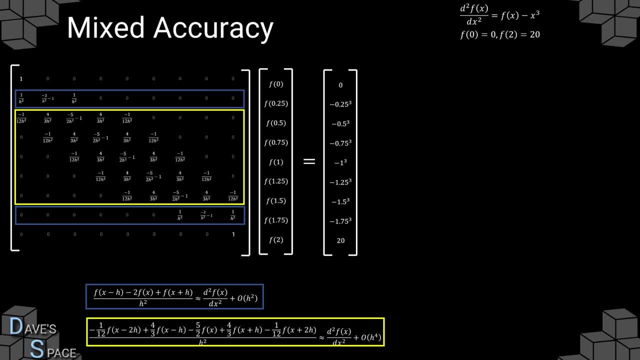 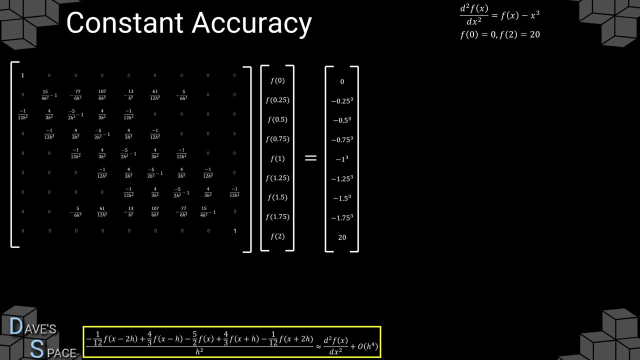 This results in the nine equations required, but means the two points next to the boundaries are no longer to the fourth power inaccuracy. So any inaccuracy at these points will diminish with step size slower than those everywhere else. Our second option was again to keep the fourth-order accuracy, central difference. 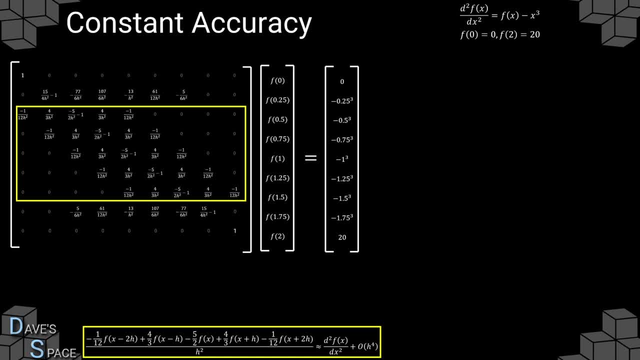 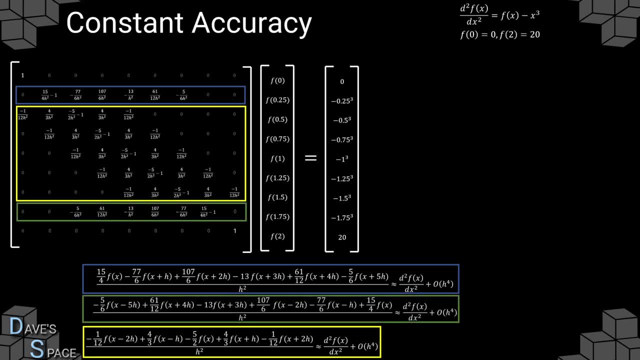 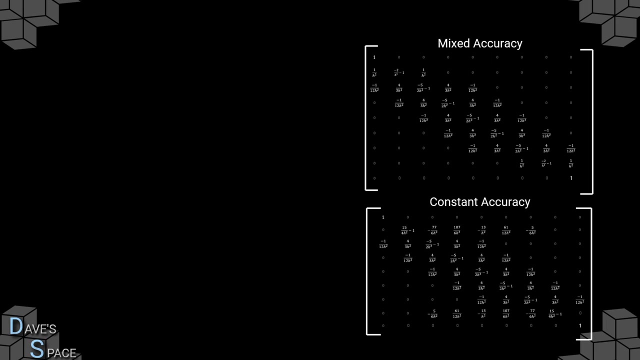 equations, But then introduce the forward fourth-order accuracy to the left edge and the backwards fourth-order accuracy to the right edge. Now, any error in the approximation is proportional to the fourth power of h everywhere that we evaluate it, And so we can summarize these as being called mixed accuracy and constant. 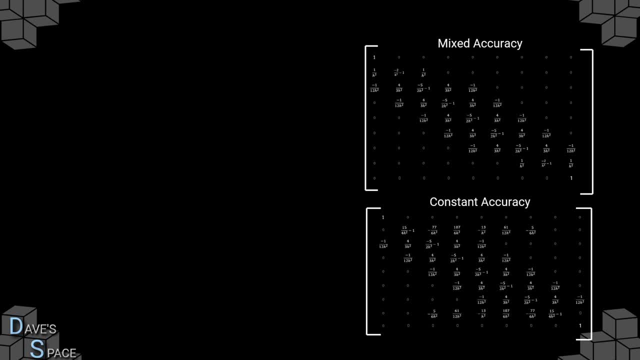 accuracy, With the mixed accuracy being, in which we reduce the accuracy of the equations at the edges and the constant accuracy, meaning we introduce forward and backwards finite difference methods when the central difference method does not fit in that row. So let's look at an even more 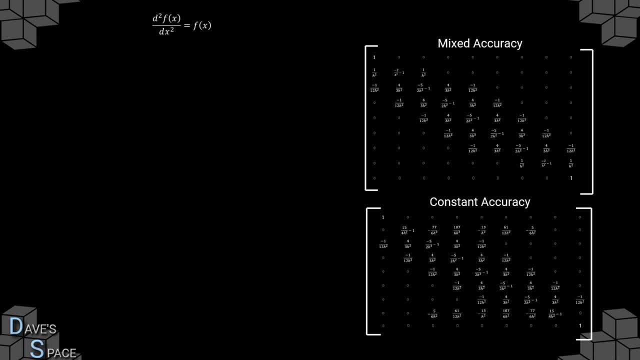 interesting example, which is the second differential: f is equal to f. The boundary conditions: f naught equals one and f2 equals e squared. The student among you may recognize shipman. many say that this is a doctors within the. You may recognise this as a differential equation describing exponential growth with an analytical 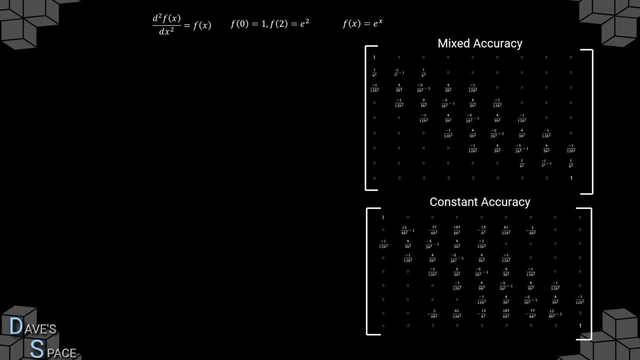 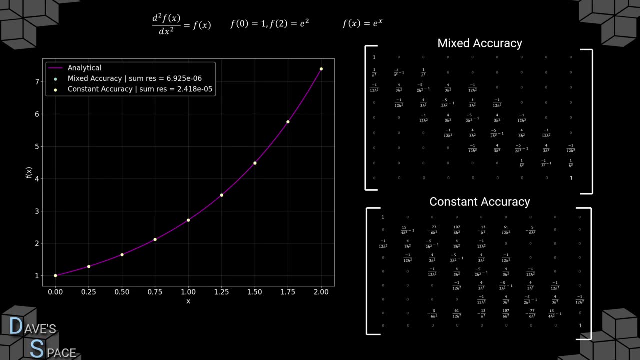 solution of f of x equals e to the x. We can solve this by using the two matrices from earlier, since the matrix is the same because in our previous equation the second derivative of f was equal to f minus x cubed. So our A matrices remain the same, but all we need to do is change the p vector. 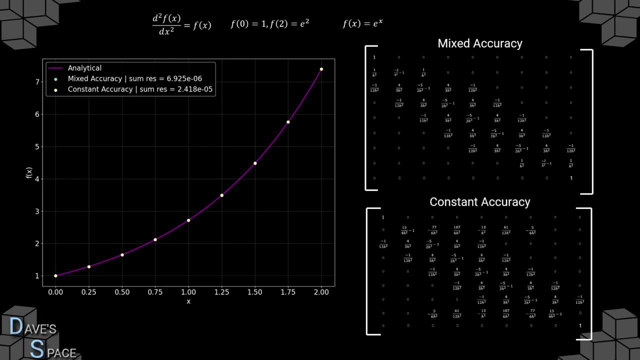 We see that both of them solve the equation visually very well. so just by looking at this plot, no differences can be seen from either method when compared to the analytical solution. A good measure of how well a numerical method performs is to calculate the sum of the squared. 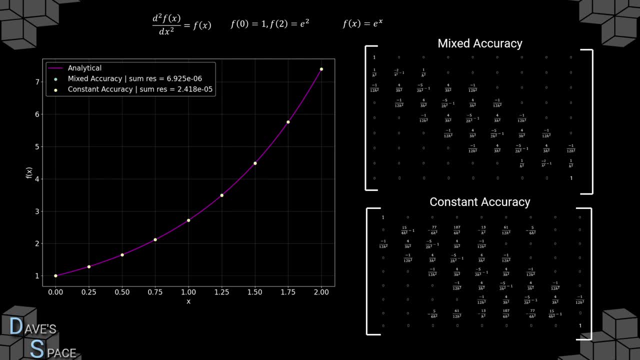 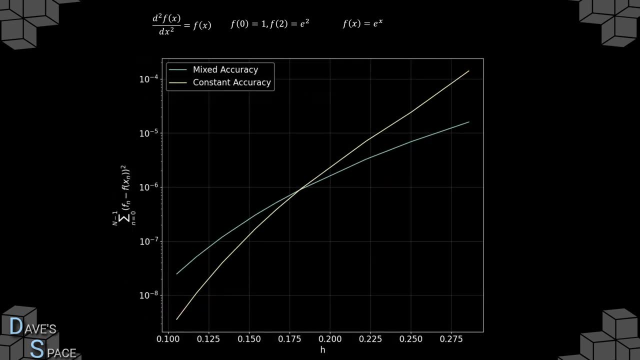 residuals. So for a function like this, in which we know the analytical solution, we can go ahead and evaluate how far each of the points is from the analytical solution and then square those values and add them all together. So this is the sum of the square residuals, which is also called the global error. 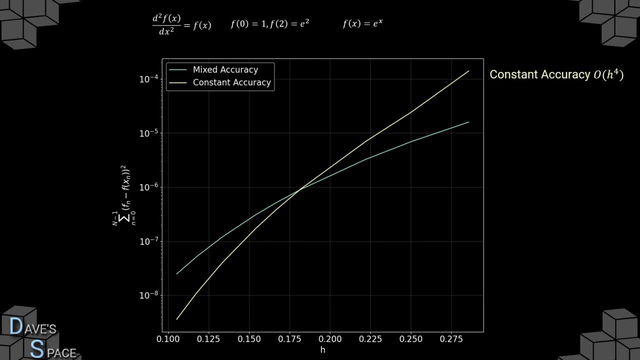 Here we can see the sum of the squared residuals, both constant accuracy and mixed accuracy. We can see the trend we observed earlier in that a smaller step size results in better accuracy, so we get a lower global error. What is interesting to see here is that the constant accuracy actually has a larger global 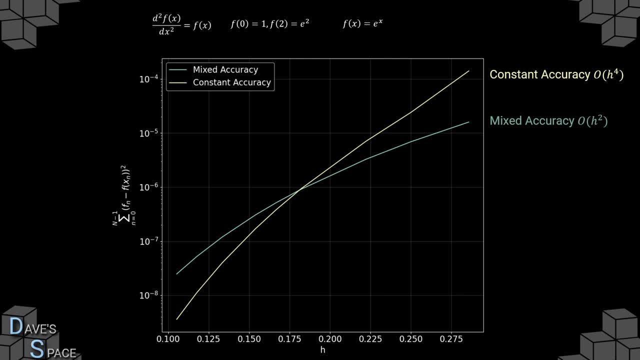 error for a larger step size. This is not too surprising, Because we know the central differences are better than the forward and backward differences, and the constant accuracy involves forward and backward differences near the edge. However, as the step size decreases, the rate at which the global error decreases is. 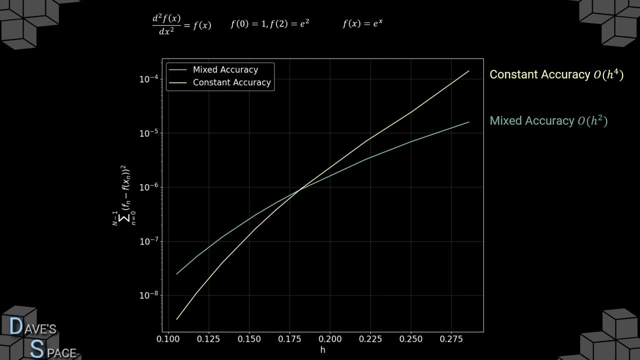 greater for the constant accuracy. since this accuracy is h to the 4 for every equation At some step size, the constant accuracy of h to the 4 results in a lower global error. So here it's a step size of around 0.. 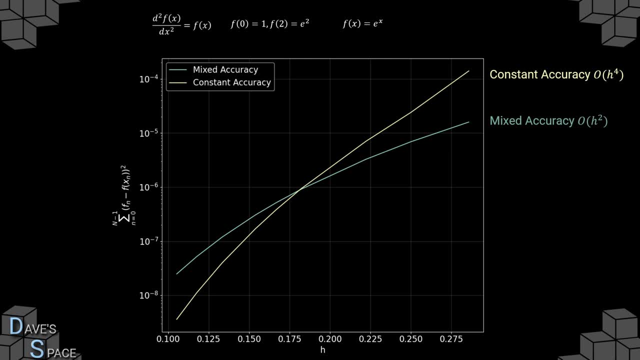 This won't always be the case. it obviously depends on the equation, And so, even though 7 out of 9 of the points are approximated with h to the 4 accuracy, the two endpoints where we reduce the accuracy to h squared will always hinder the global. 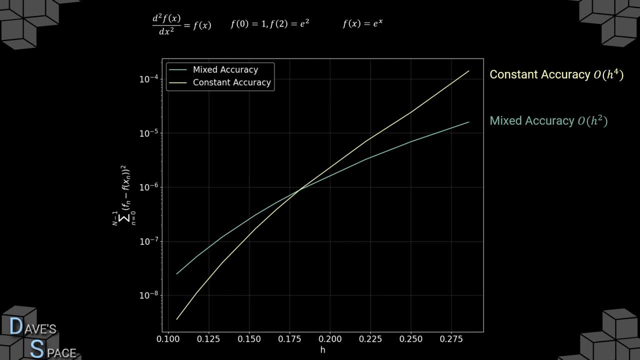 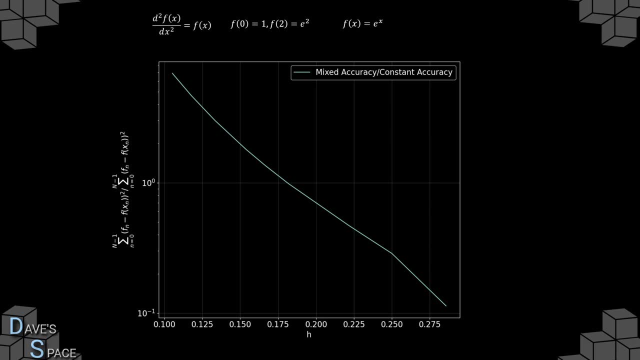 error when using mixed accuracy. And if we look at the ratio between the two, we can see that smaller step sizes favour the constant h to the 4 accuracy. As the h squared decreases, the constant h to the 4 accuracy increases. So h squared accuracy just can't keep up. 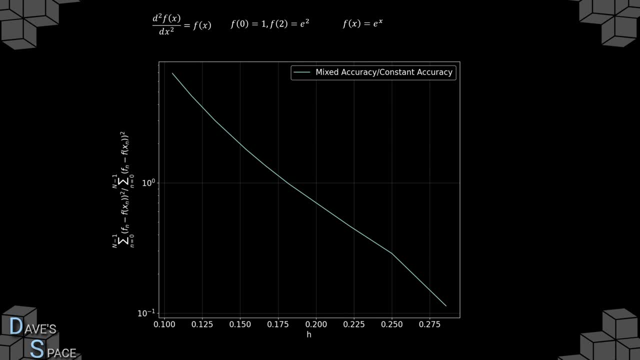 Where the transition occurs, which we said was around 0.18, will rarely be known as the differential equation to solve, may not have an analytical solution, And so it's a key point of the finite difference method is that a method is only as good as